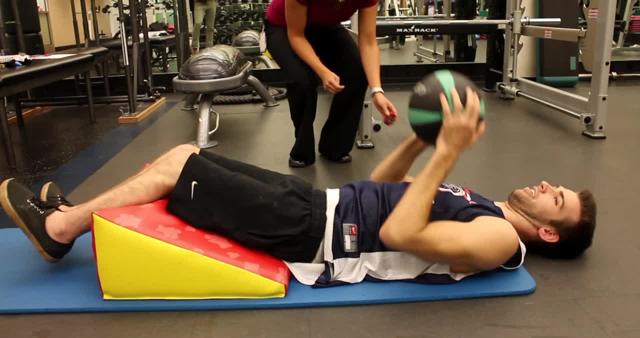 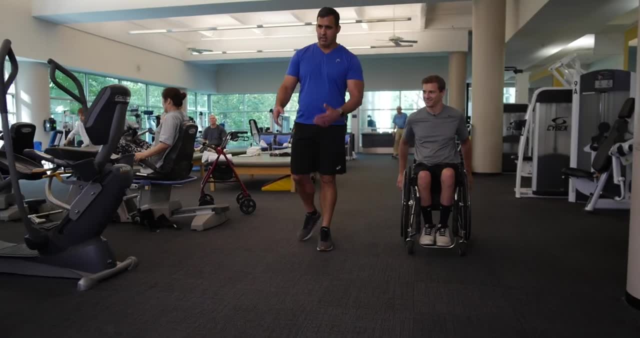 strength training. they can help you stay focused and be the voice reminding you to slow down and control your movements. Number three: dress appropriately. While working out, you should dress in a manner that is both comfortable as well as helpful. That means choose something that moves. 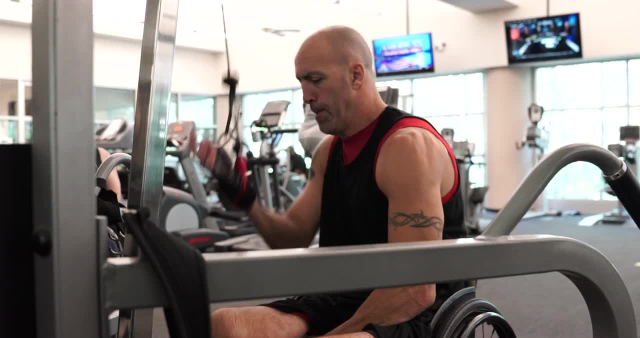 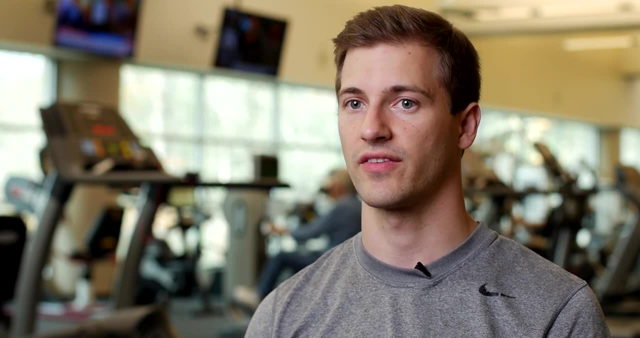 easily and does not restrict your range of motion, as well as something that breathes so you won't get hurt. Number four: wear a tight fit. Dry fit clothing is a great material to exercise in, because it wicks the sweat from your body and allows you to stay cooler. Avoid wearing jewelry. 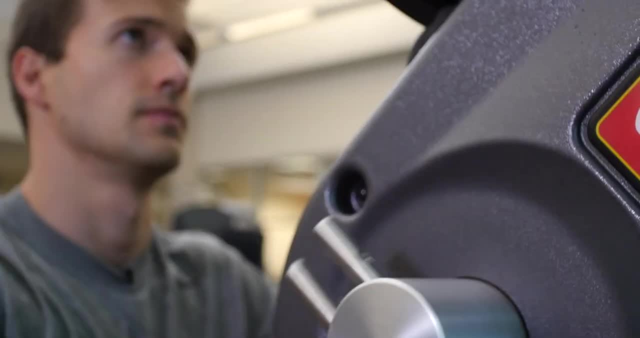 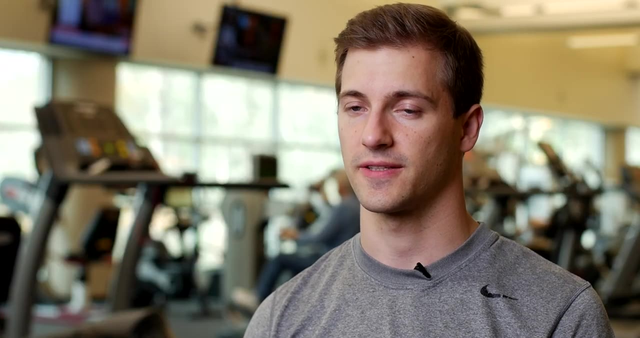 or necklaces that can get caught on exercise equipment and cause injury. You should also take into account what type of exercises you'll be doing, as well as the environment you'll be in, as that may also influence your clothing choices. Number four: use correct form. Using correct form. 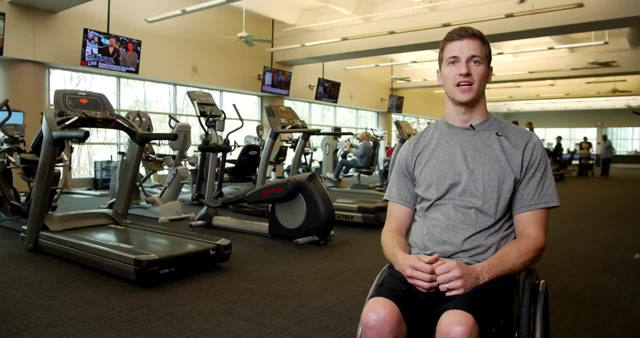 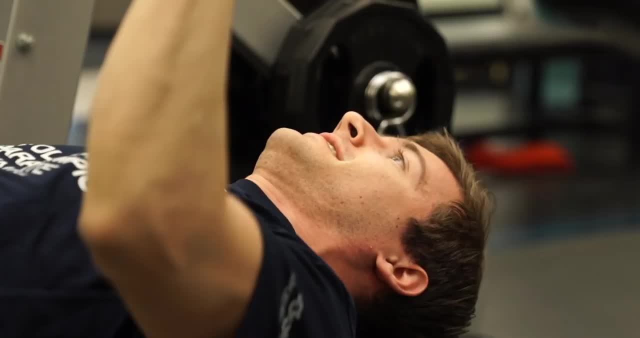 will not only allow you to focus on getting the most of each movement, but will also help prevent injury. Starting with weights, you'll be putting stress on your joints and tendons. Staying mindful to use the correct motions will prevent you from putting any undue stress on these areas and reduce 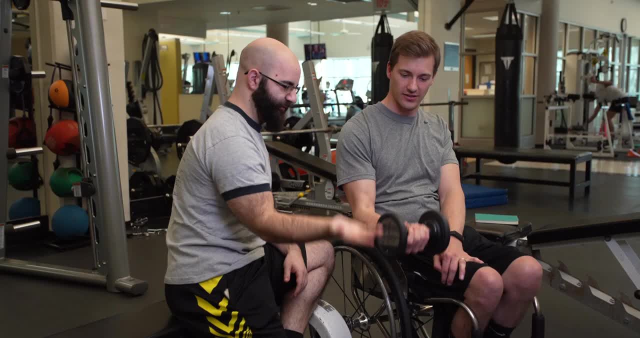 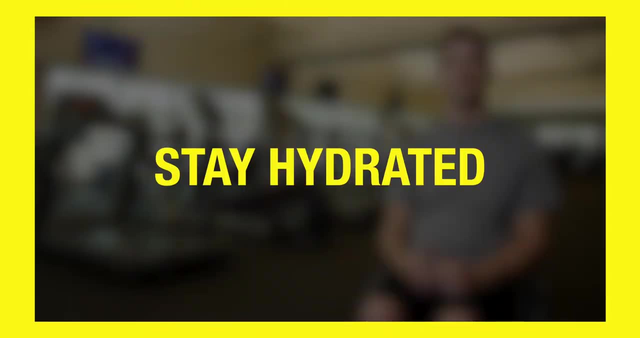 the risk of injury. Another key in knowing what form will work best for you is to meet with a trainer who knows the human body well enough to adapt movements for you based on your mobility. Number five: stay hydrated. Drink water before, during and after your workout. Dehydration can 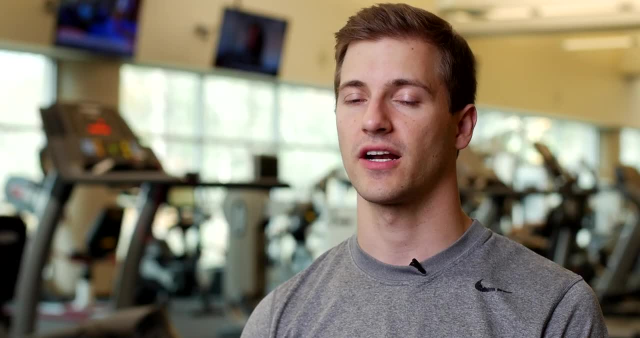 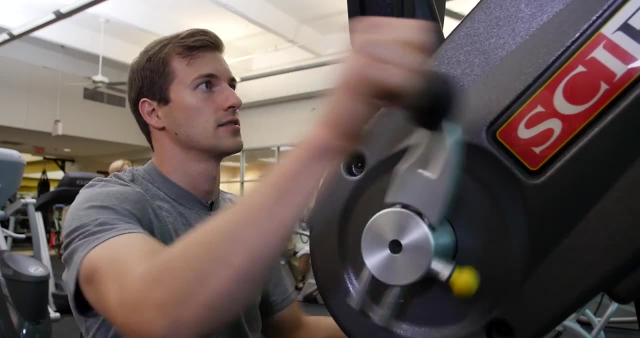 not only lead to fatigue, dizziness and confusion, but can also result in heat injuries, such as heat strokes and other serious health issues. As you work out, your body is going to heat up, which means you're going to sweat, So it's 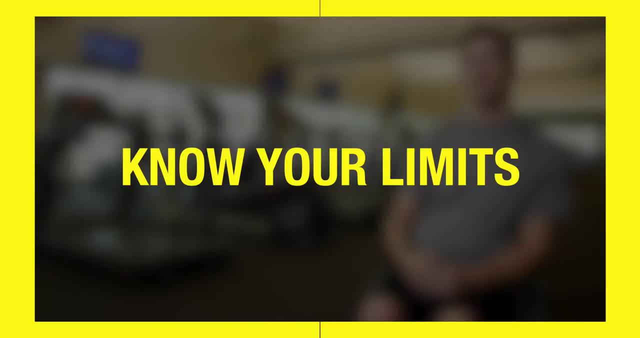 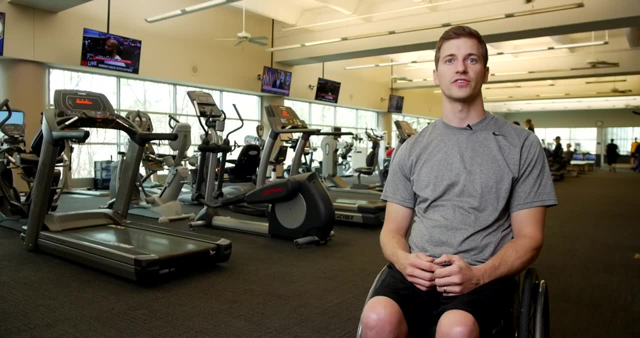 important to drink plenty of fluids, especially water. Number six: know your limits. It's important to push yourself, but it's just as important not to push yourself too far. Overdoing it can lead to injury and burnout. so it's good to be aware of your current level of fitness. Some fitness: 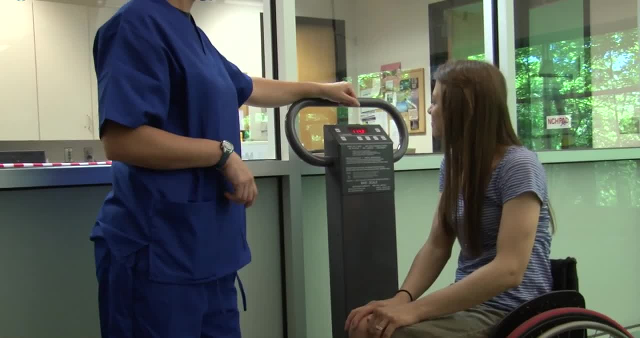 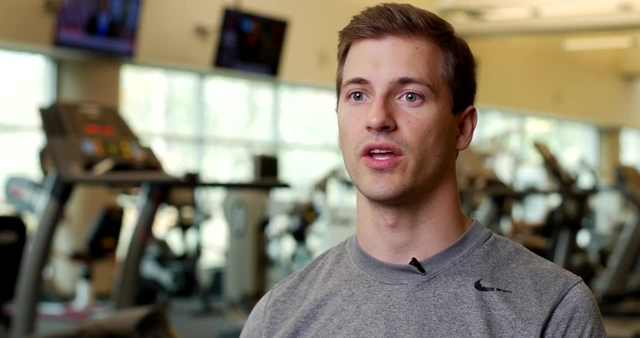 centers offer health assessments that can give you an idea of what level you're starting at. Having this information will help you when determining where your limits are. If you do go too far, your body will tell you what you need to know. It's your job to listen, so be sure to.